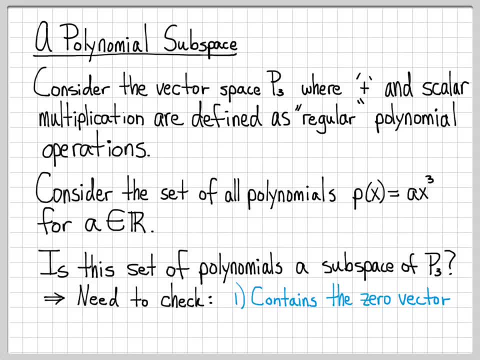 to check three things: I need to check that our subspace contains the zero vector. I need to check that it's closed under addition. And I need to check that it is closed under scalar multiplication 0- 0- three properties. then this set is a subspace of the vector space P3.. And since it's a subspace, 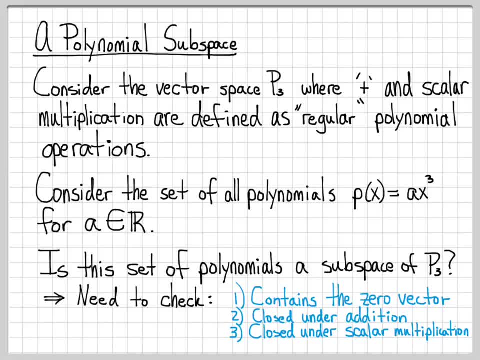 it's itself a vector space. All the other properties, the other seven properties that we won't check explicitly, those are all inherited from P3 in a trivial way that we don't even need to check for. So let's go ahead and see if this set of polynomials of the form ax cubed for. 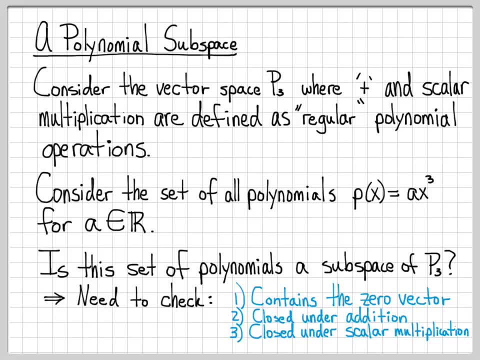 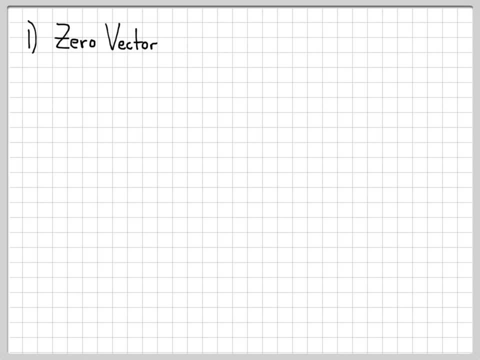 arbitrary values of a in the reals is indeed satisfying these three properties. So let's go through them one by one. So, first of all, does this collection of vectors contain the zero vector? Note that I get to choose any value that I want in a. So for all, a in the reals. that means I can: 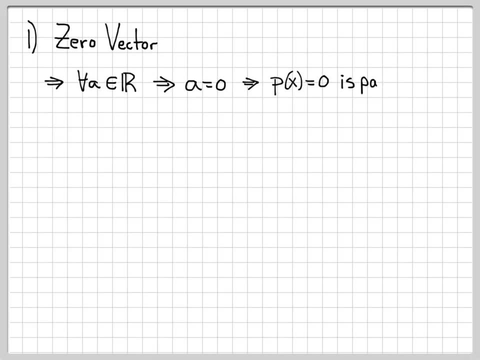 let a equal zero. So that means that my set contains the polynomial P of x equals zero. This is one of the vectors in this set. That means that for any P of x that I want to choose, so for some arbitrary P of x in my set, if you want to. 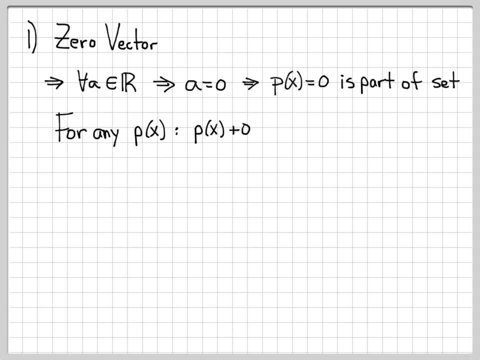 think of that as bx cubed or 1.2x cubed or a2x cubed. I can add zero to it and end up back where I started. So this element P of x equals zero satisfies exactly the zero property that. 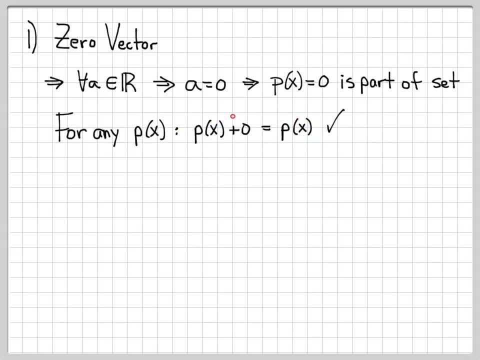 I need Any arbitrary P of x that I choose. when I add this zero element to it, I get back where I started. So this is part of the set and it satisfies the zero property. So I can put a zero vector property. What about being closed? under addition, Let's choose two arbitrary. 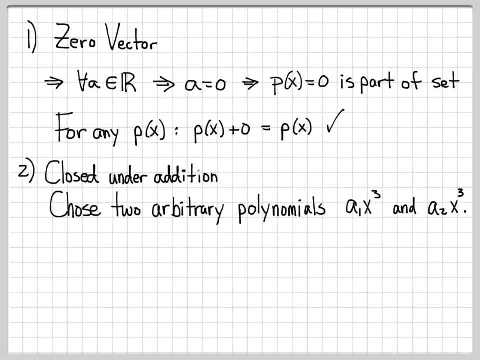 polynomials from the set that I'm working with. So let's choose a1x cubed and a2x cubed. So these are both elements of my set and I've chosen them very arbitrarily, letting a1 be an arbitrary number and a2 be an arbitrary number from the reals. Let's see what happens when I add them.